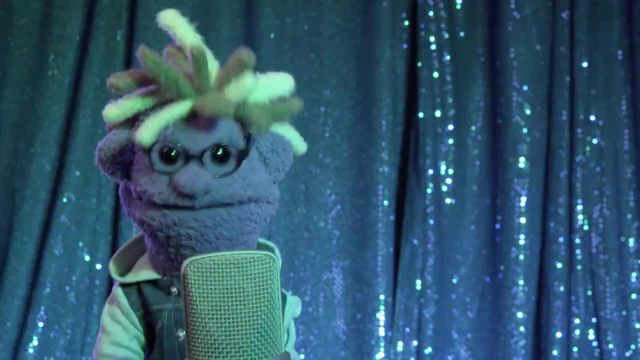 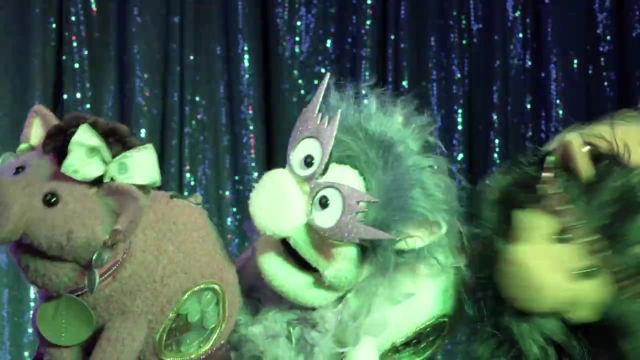 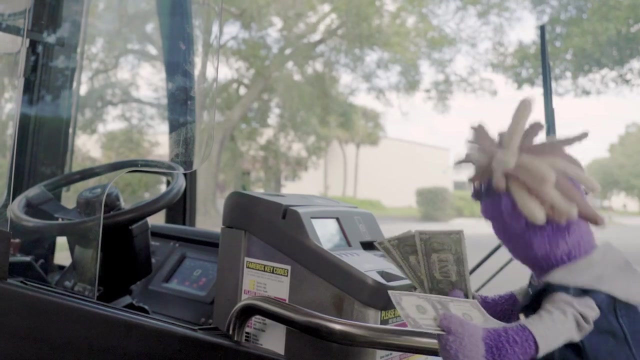 Dance to a jam as I reminisce, and it went a little something like this: Saving spending, sharing budget, Saving spending, sharing budget, Saving spending, sharing budget. Look out, Jay, here comes payday Money in my hand without a care. I jumped on the. 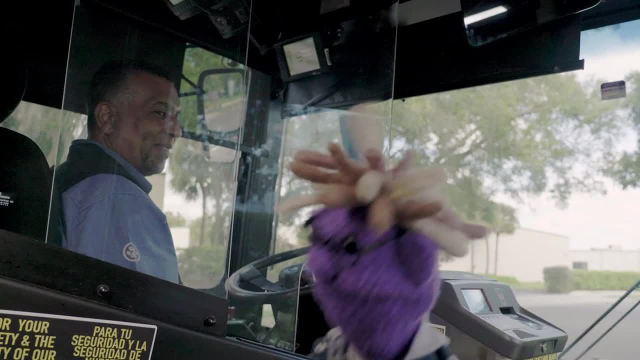 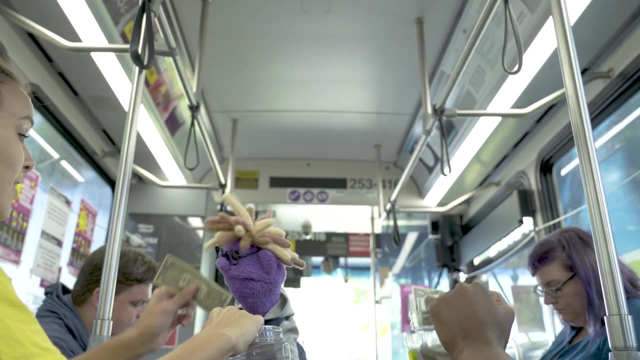 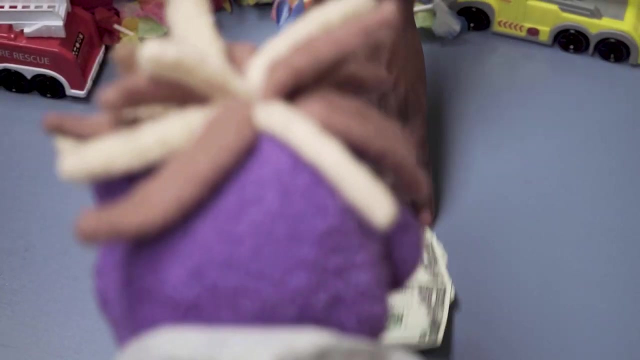 bus and paid the dollar fare, Rolling downtown feeling like a big man. People ask for my help. I put money in their hand. You need help with this, I can help with that. You need help with this, I can help with that. Up on the boogie step, step into the store, Yep, slam My money on. 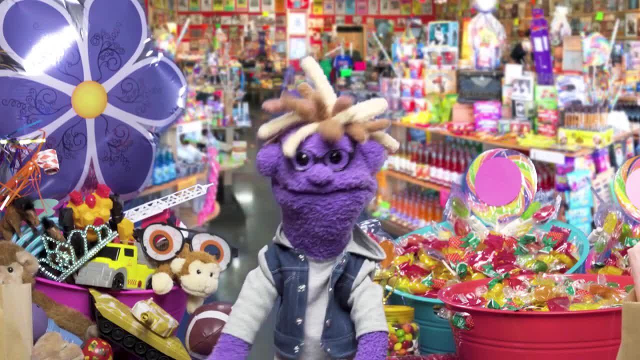 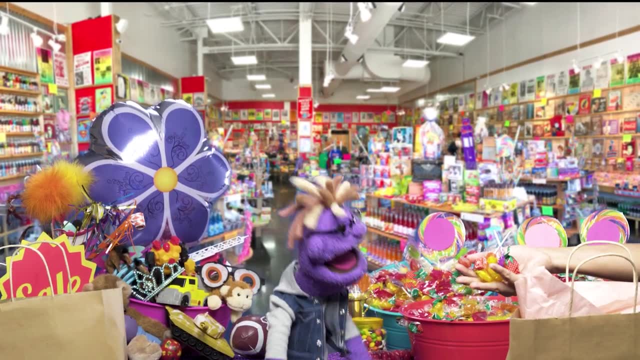 the counter and I'm feeling good because I'm the king of this neighborhood. I don't need to see the tag, sir. Just put it in the bag, sir, Just put it in the bag. More toys- Put it in the bag. 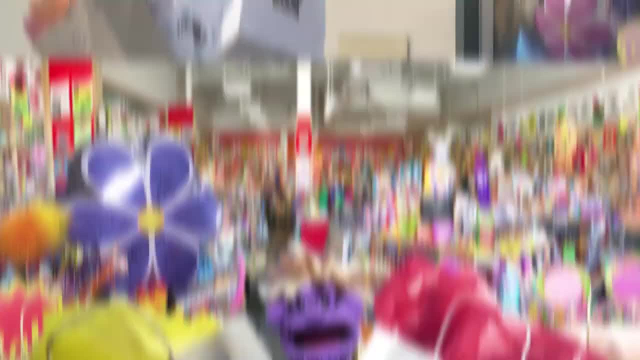 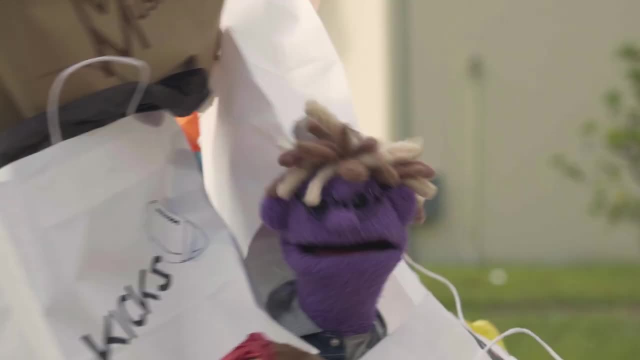 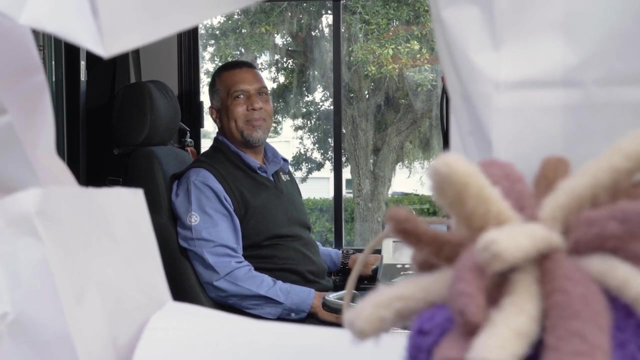 And what about this? Just put it in the bag. Okay, I've got bags full of goodies, but my pockets are bare And, uh-oh, I can't pay the dollar fare. Sorry, Jay, if you can't pay, you'll have to get home another way, Stranded on the corner. 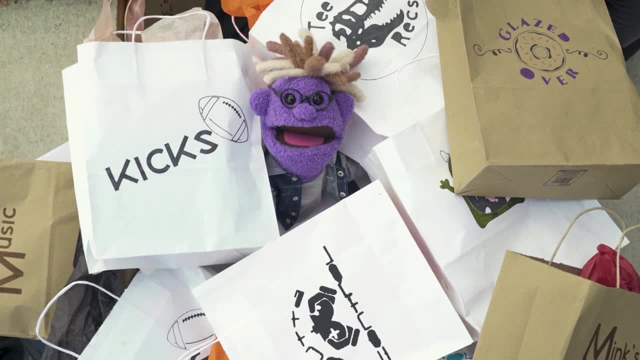 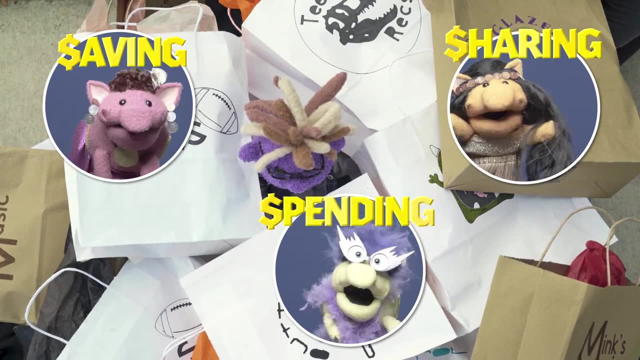 with a frightened thought. I don't even know what I just bought. Saving spending sharing budget. Saving spending sharing budget. Saving spending sharing budget. Work hard Jay, spend pay one day. Saving spending sharing budget. Saving spending spending budget. Work hard Jay, spend pay one day. Saving spending sharing budget. Saving spending spending budget: Work hard, Jay, spend pay one day. Saving spending sharing budget: Work hard, Jay, spend pay one day. I know where I was the third week in. 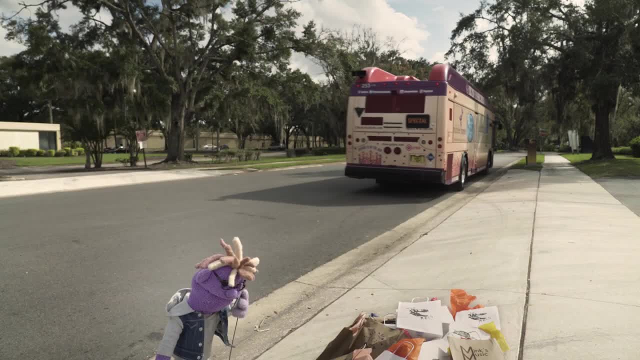 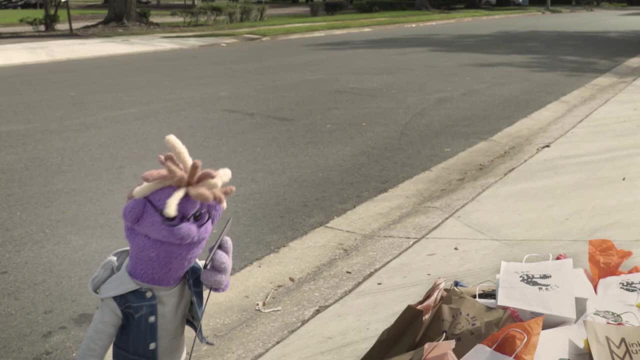 the row Stranded on the corner. having spent my dough, I called my mom. hey, I straight messed up. She said I'll be right there to pick you up. Sorry, mom. Yeah, yeah, yeah, I'm on the corner. 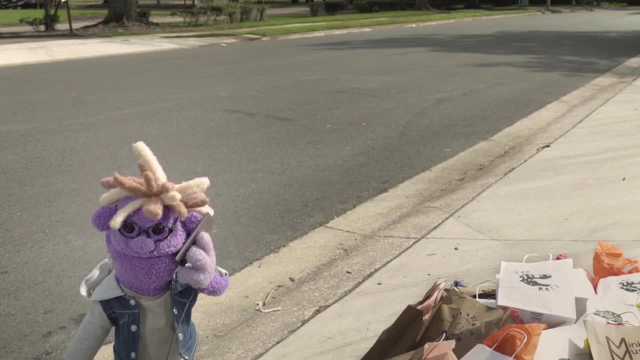 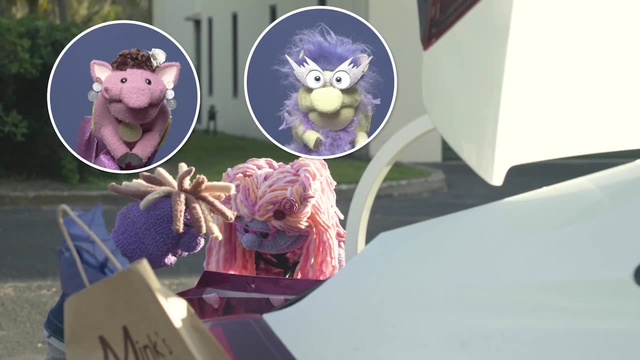 Yeah, right, right again. When mom saw my bags, I thought she would nag, But instead she gave me a bag Inside three piggy banks- cute as a nugget, She said. these will help you to make a budget. I 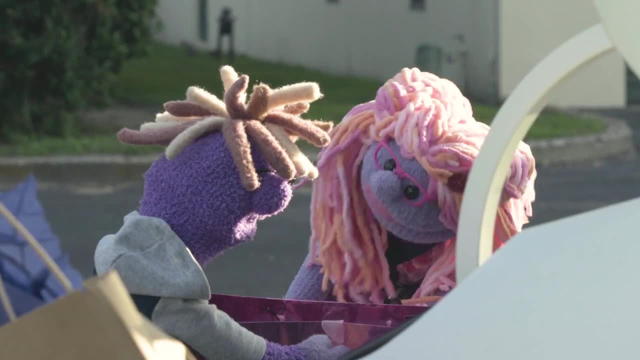 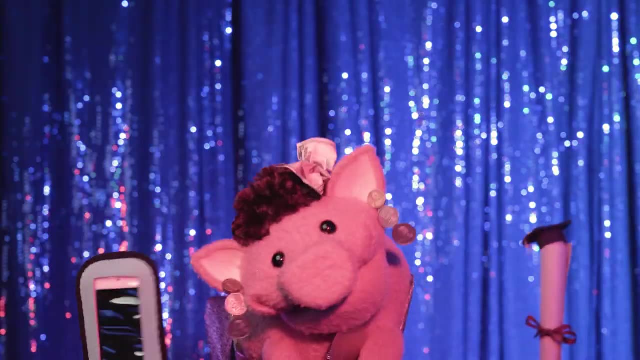 said: what is that? And she said: honey, a budget is a plan of how you use your money. I'm the first little piggy. I'm used to save. I hold money for big things you want one day, Whether electronics, college or a bike- to steer Your savings. money goes in here. Feed a little each week. 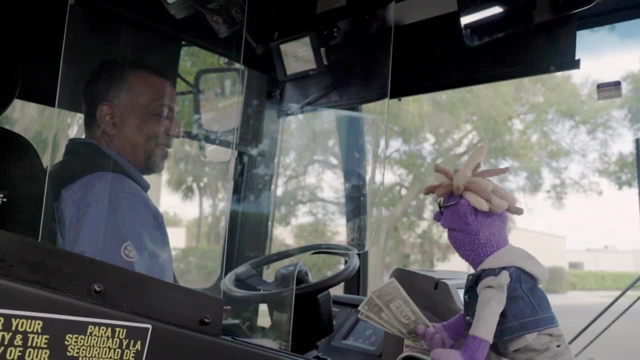 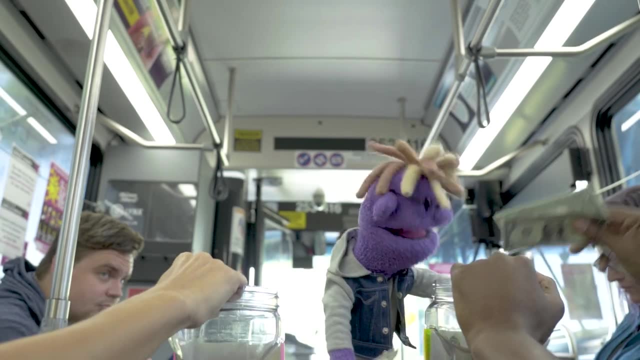 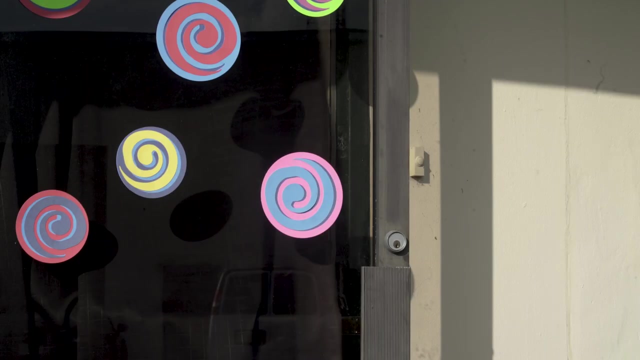 without a care. I jumped on the bus and paid the dollar fare, Rolling downtown feeling like a big man. People ask for my help. I put money in their hand. You need help with this, I can help with that. You need help with this, I can help with that. Up on the boogie, Step, Step Into the store, Yep. 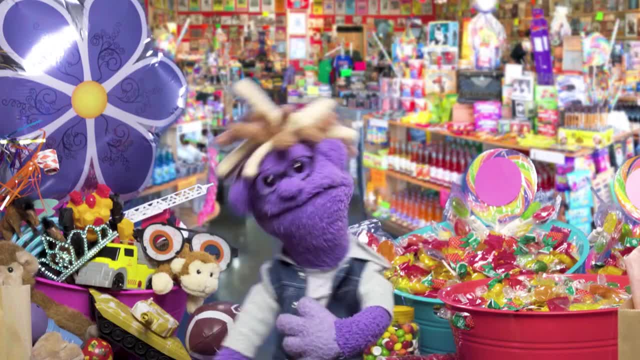 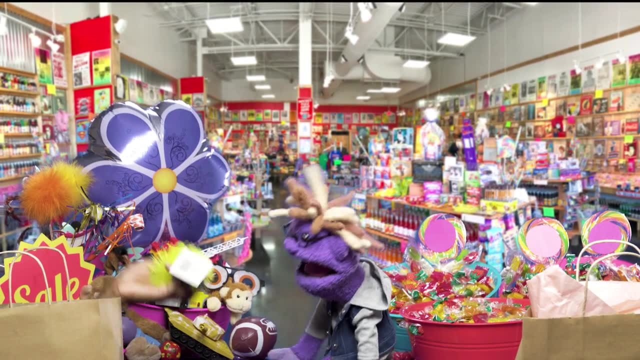 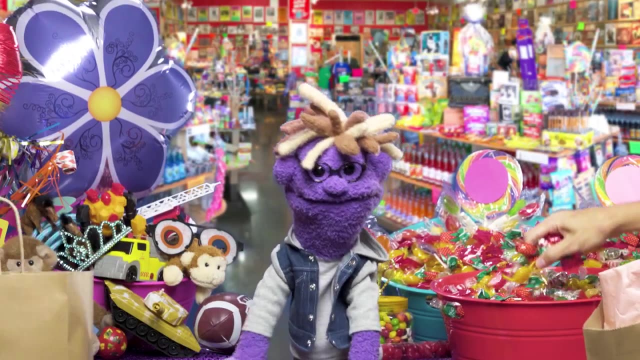 Slam My money on the counter and I'm feeling good cause I'm the king of this neighborhood. I don't need to see the tag, sir. Just put it in the bag. Just put it in the bag. More toys, Put it in the bag. And what about this? Just put it in the bag, Okay. 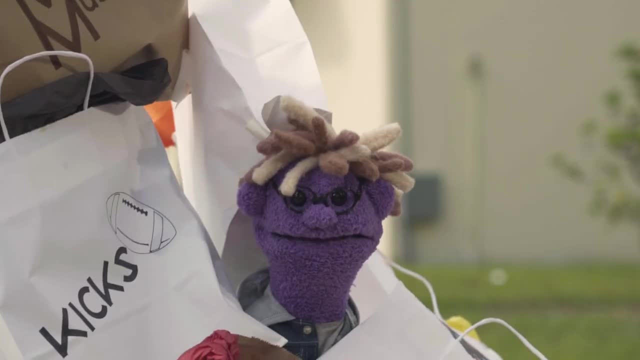 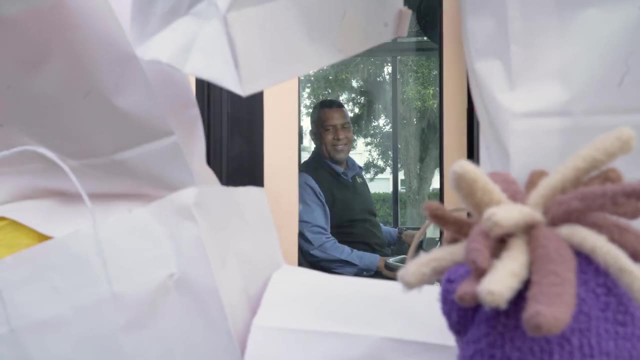 I've got bags full of goodies but my pockets are bare and, uh-oh, I can't pay the dollar fare. Sorry, Jay, if you can't pay, you'll have to get home another way, Stranded on the corner with a frightened thought. I don't even know what I just bought. Savings Spending Sharing Budget. 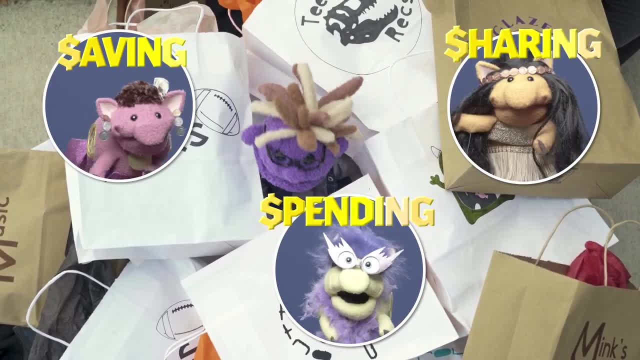 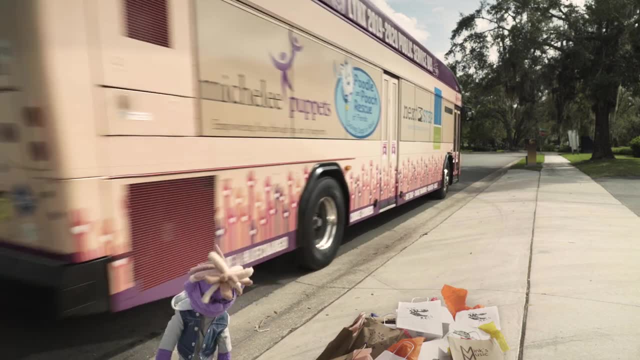 Savings Spending- Sharing Budget. Savings Spending- Sharing Budget Budget. Where Ty Jay spent pain one day. There I was the third week in the row Stranded on the corner, having spent my dough. I called my mom- Hey, I straight messed up. She said I'll be right. 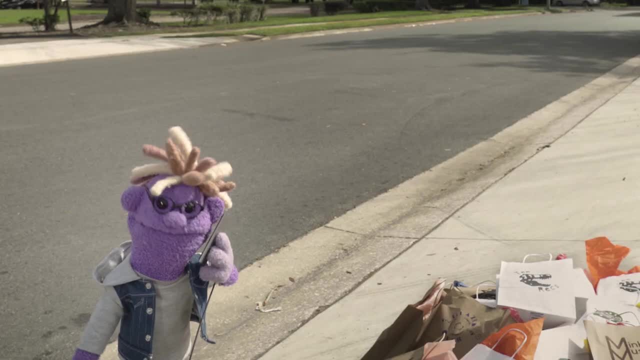 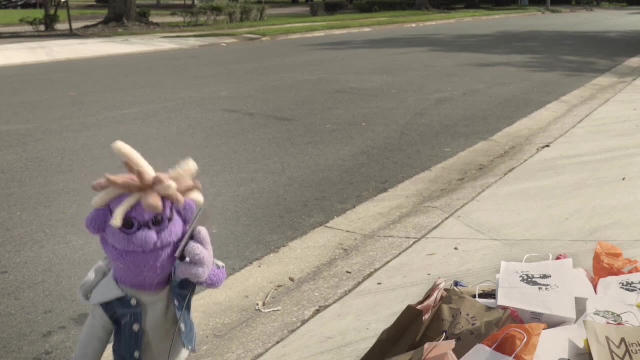 there to pick you up. Sorry, mom, Yeah, Yeah, Yeah, I'm on the corner. Yeah, Right, Right Again. When mom saw my bags, I thought she would nag, but instead she gave me a bag Inside three piggy. 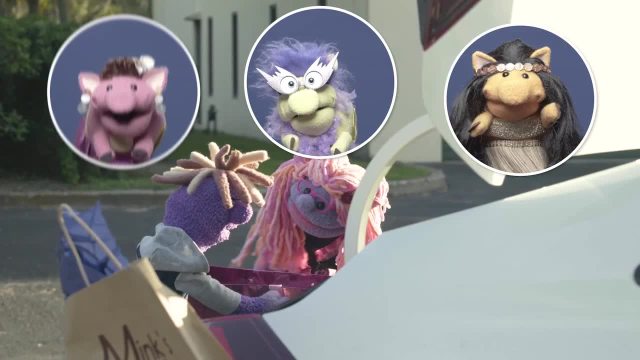 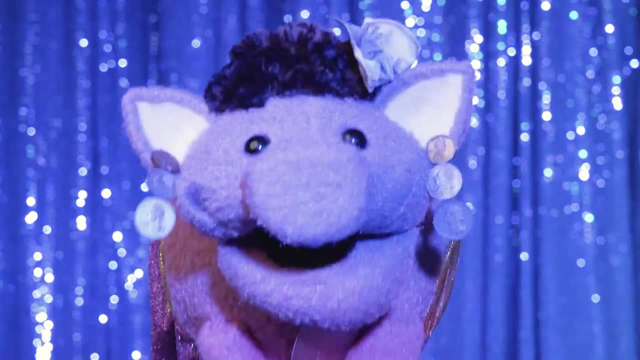 banks. cute as a nugget. she said these will help you to make a budget. i said: what is that? and she said, honey, a budget is a plan of how you use your money. i'm the first little piggy. i'm used to save. i hold money for big things you want one day, whether electronics, college or a bike to steer. 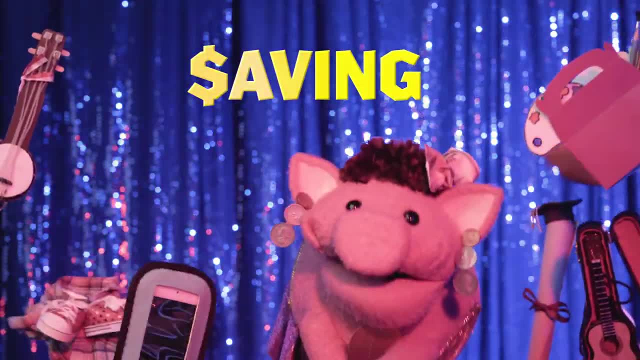 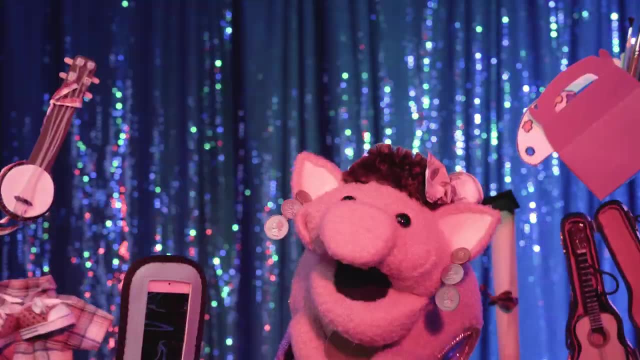 your savings money goes in here. feed a little each week. it adds up a lot soon you won't believe how much money it got. but if you're looking for money to use every day, my son and sisters got you jay. i'm the second little piggy. i'll be your best friend. just feed me the money you want to spend. 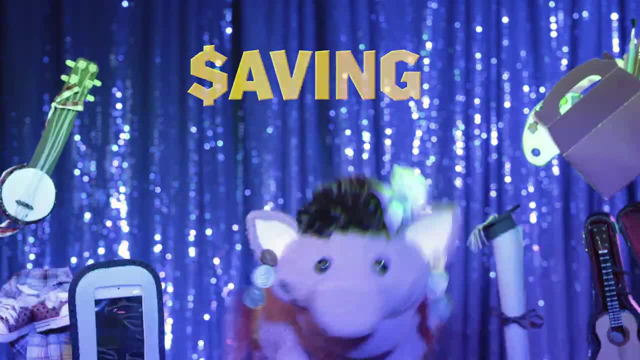 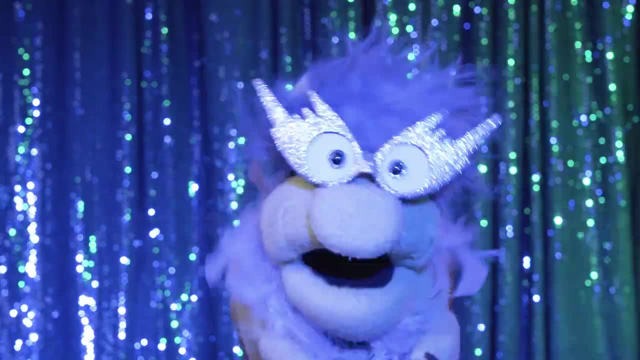 it adds up a lot. Soon you won't believe how much money it got. But if you're looking for money to use every day, my spending sister's got you. Jay, I'm the second little piggy. I'll be your best friend. Just feed me the money you want to spend For daily things. 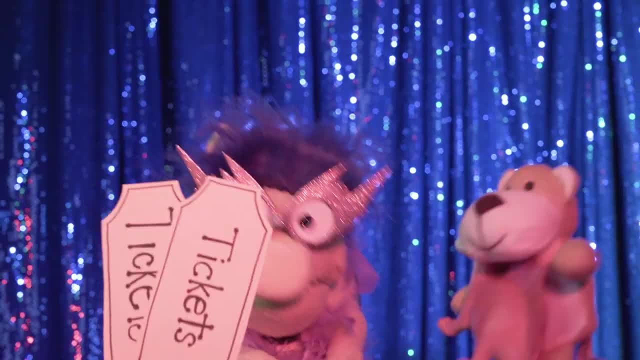 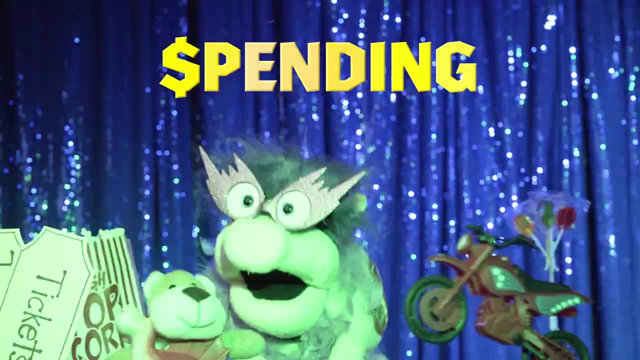 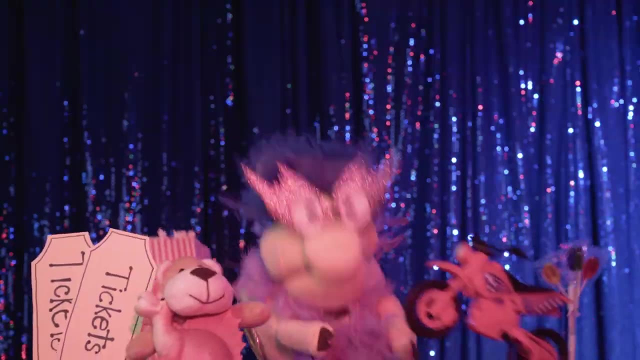 you want to do, I'll have the cash. that goes with you When you need cash to have some fun. spending piggy gets the job done. Need some money Pour your food? Don't worry, Jay, I got you dude, But for money used. to show you care, let me introduce you to my girl, Cher. 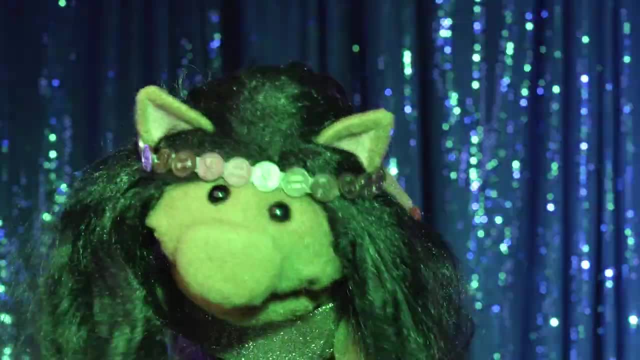 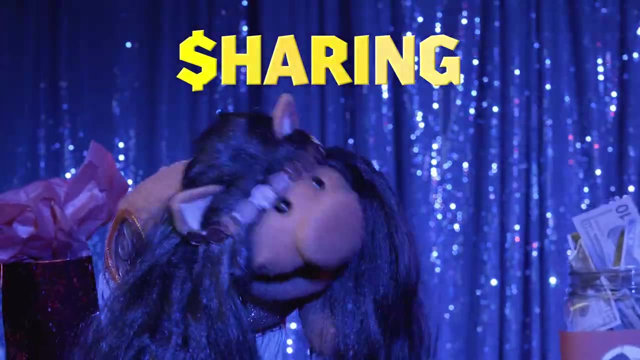 My name is Cher, with hair down to there. I help collect money that you can share. If there's a cause you want to support, like building a field for your favorite sport or buying a present for your best pal, I'm the second little piggy. I'll be your best friend. Just feed me the money you want. 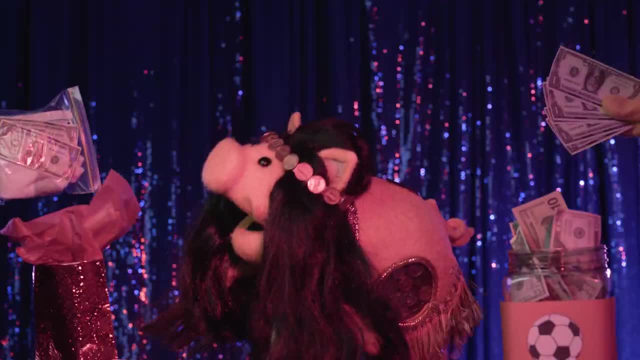 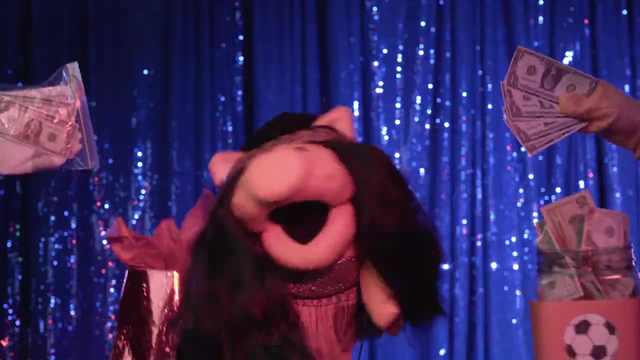 to spend For daily things. I'll have the cash that goes with you When you need cash to have some fun sharing. piggy is your gal. A dollar here, a dollar there helps the world. when you share, Working together, we can make change. Jay, don't worry, I got you babe. 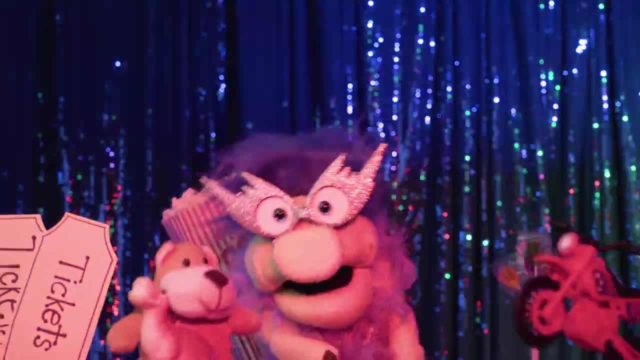 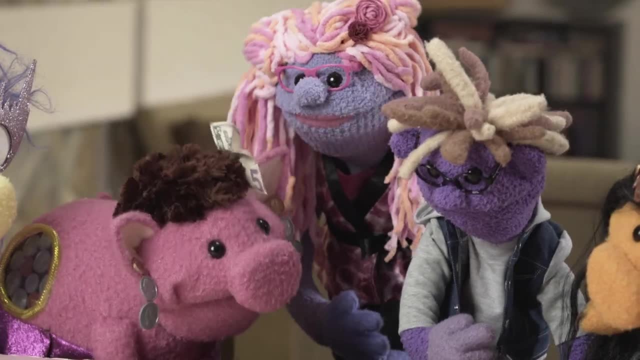 Saving Spending, Sharing Budget. Saving Spending, Sharing Budget. Saving Spending, Sharing Budget. Come on, Jay, let's start today. I knew those piggies and my mom were right, so we sat down and made a budget that night. If I save all my money for three weeks, 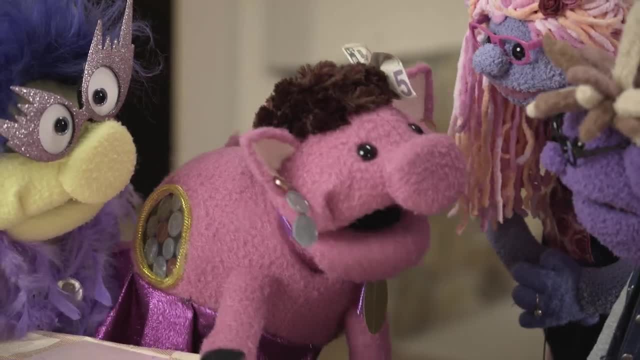 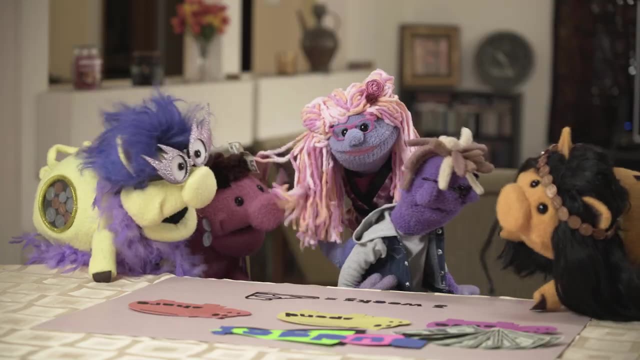 I can buy this pair of light-up sneaks, But what about my girls? They're hungry too. You won't have sharing spending money for you. A budget's meant to split your pay. We're hungry piggies. please feed us. Jay Mom said: wow, those piggies are looking at you. so what do you think that you? 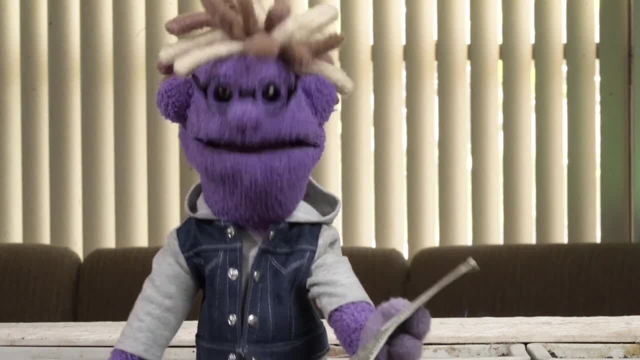 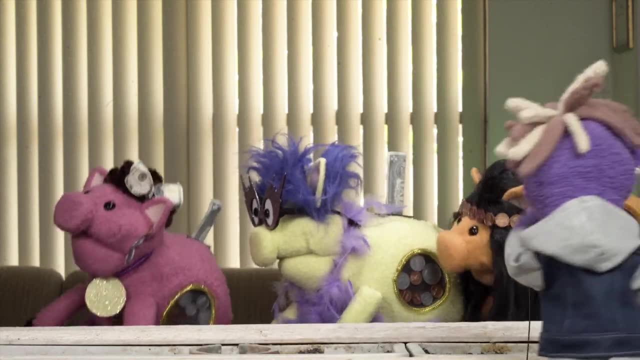 need to do. I got to spread my money among the three. I guess that's what a budget is supposed to be: Saving Spending, Sharing Budget, Saving Spending, Sharing Budget, Saving Spending, Sharing Budget. Good job, Jay, you're doing great. 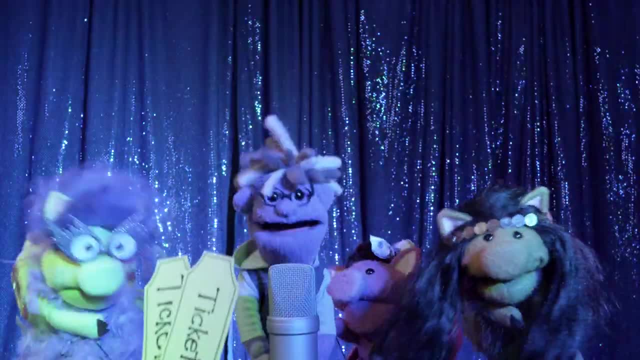 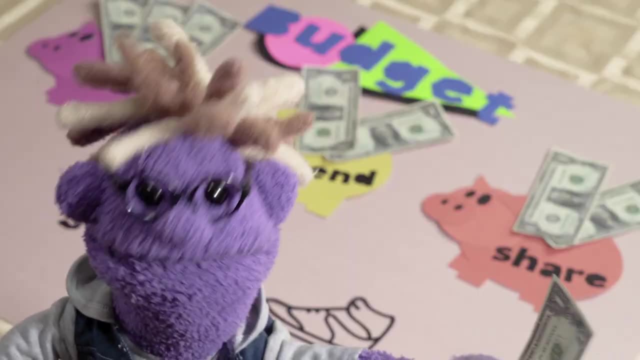 Now it's your turn. Give it a try. Plan for the things that you want to buy. Put some aside for the greater good to share with those in your neighborhood. Your budget is a plan you make today to help use your money in a smarter way. 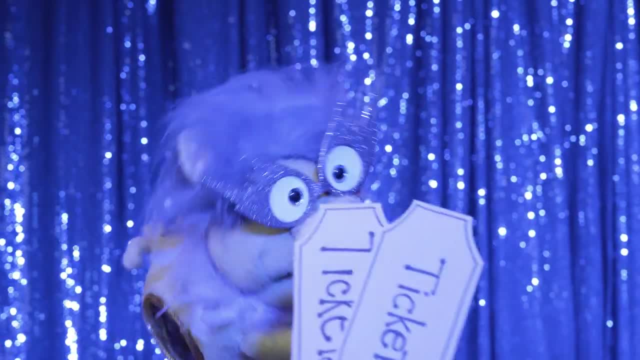 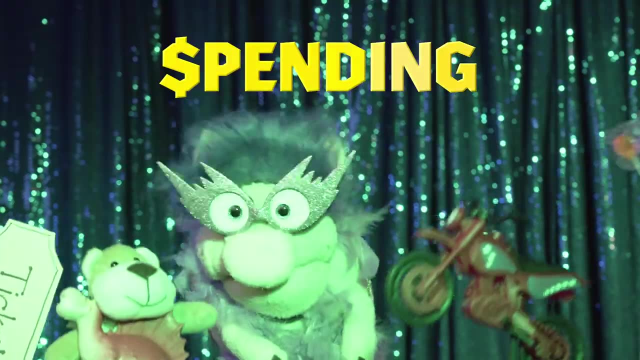 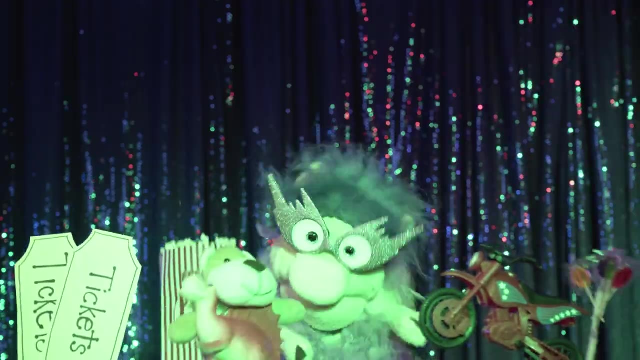 for daily things you want to do, i'll have the cash that goes with you when you need cash to have some fun, spending piggy gets the job done. need some money for your food? don't worry, jay, i got you dude. but for money used to show you care, let me introduce you to my girl. share my 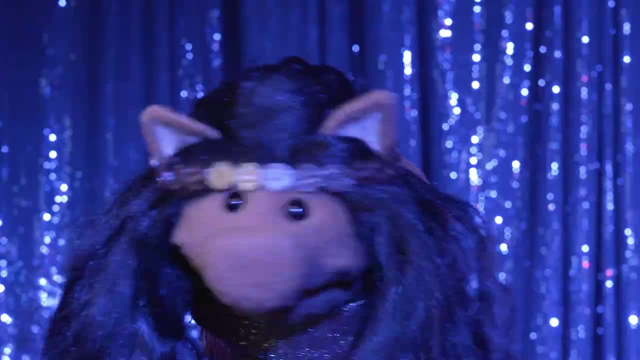 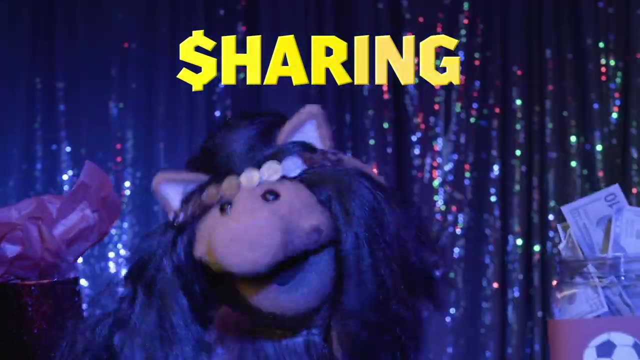 name is share with hair. down to there, i help collect money that you can share. if there's a cause, i'll be your best friend. just feed me the money you want to spend for daily things you want to support, like building a field for your favorite sport or buying a present for your best pal. 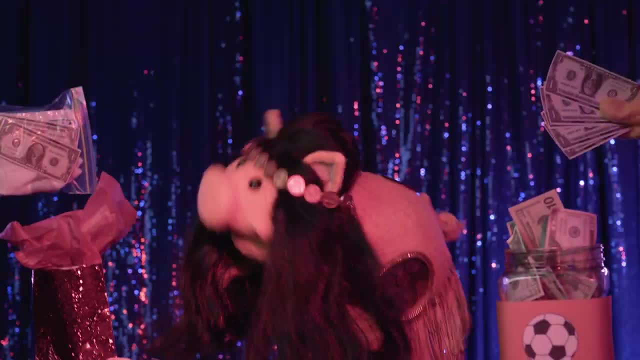 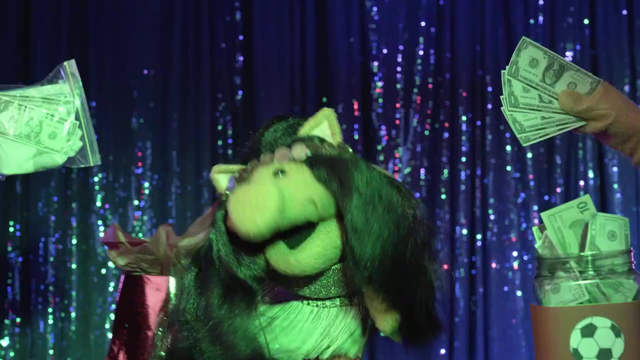 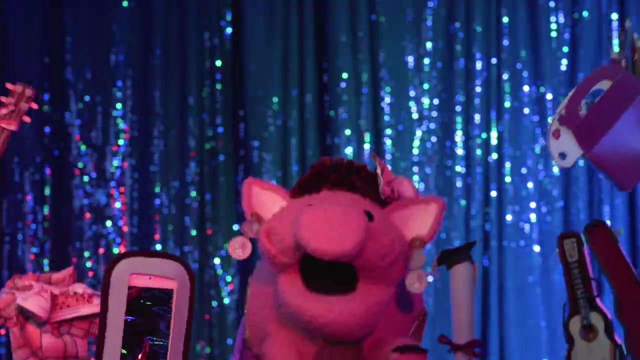 sharing, piggy, is your gaff. a dollar here, a dollar there, helps the world. when you share, working together, we can make change. jay, don't worry, i got you baby. saving spending, sharing budget, saving spending, sharing budget, saving spending, sharing budget. come on, jay, let's start. 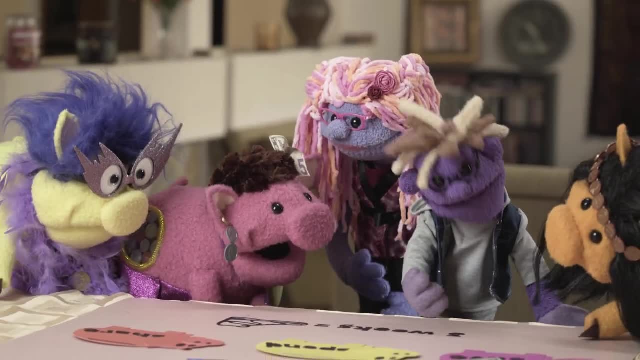 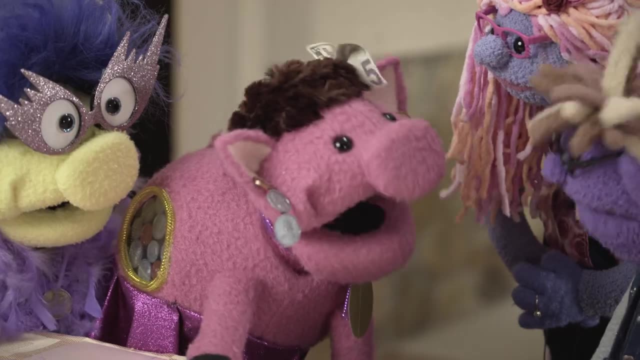 today. i knew those piggies and my mom were right you. so he sat down and made a budget that night. if i save all my money for three weeks, i can buy this pair of light up sneaks, but what about my girls? they're hungry too. you won't have sharing spending. 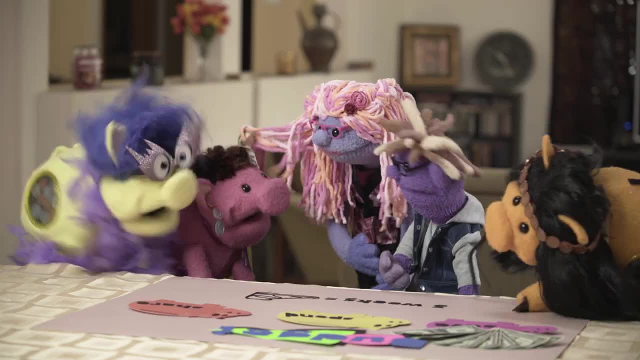 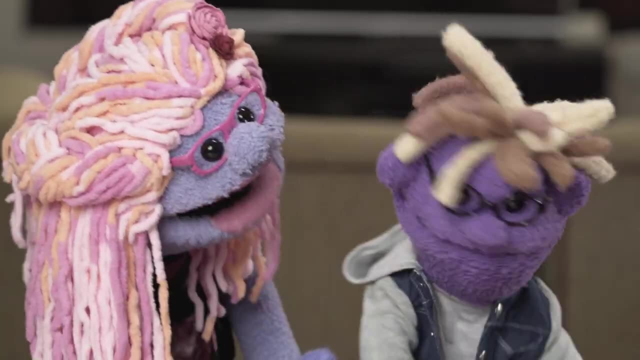 money for you. a budget is meant to split your pay. we're hungry piggies, please feed us. jay mom said: wow, those piggies are looking at you. so what do you think that you need to do? i got to spread my money among the three. i guess that's what a budget is supposed to be. 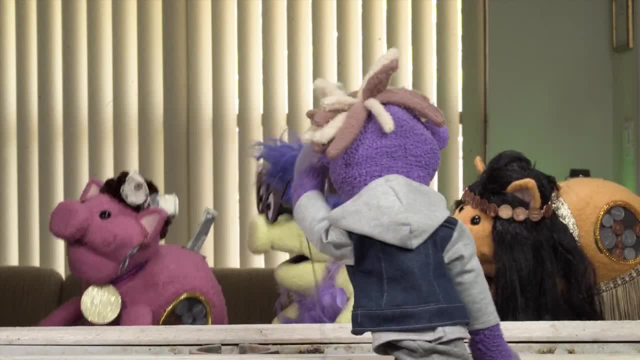 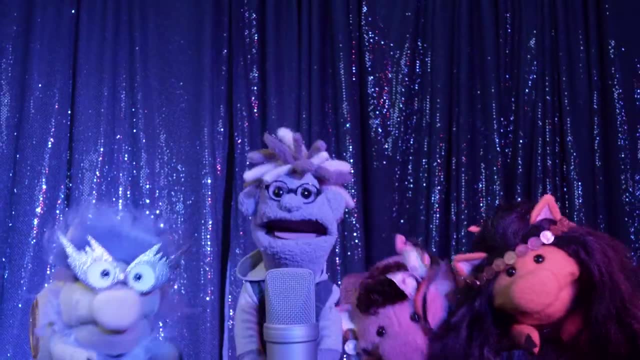 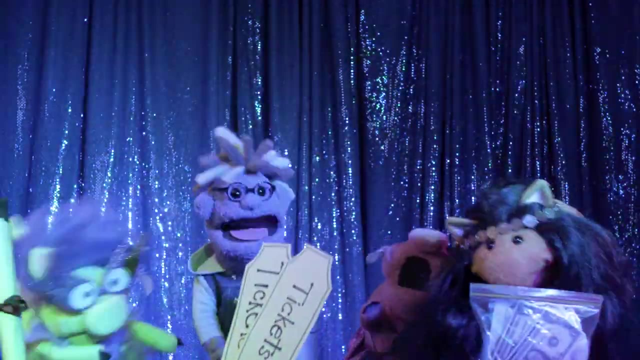 saving spending, sharing budget. saving spending, sharing budget. saving spending, sharing budget. good job, jay. you're doing great. now it's your turn. give it a try. plan for the things that you want to buy. put some aside for the greater good to share with those in your neighborhood. your budget is a plan you make today to help use your. 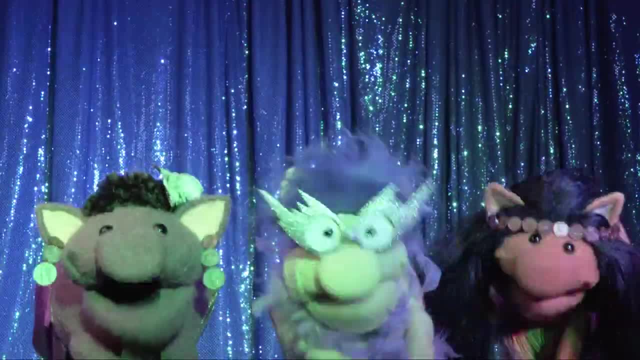 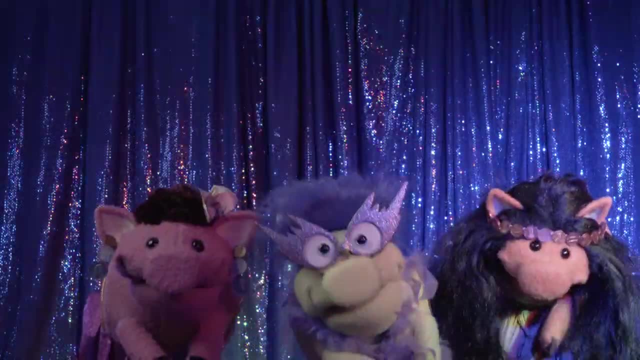 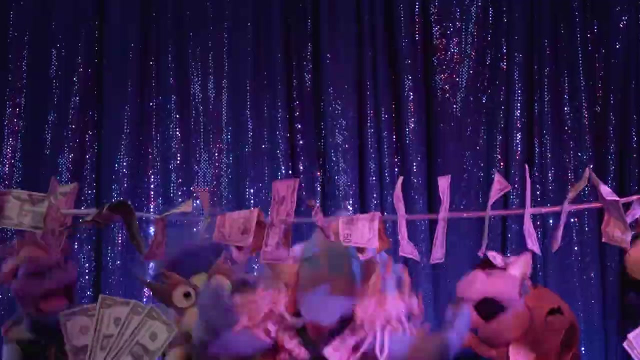 money in a smarter way: spending sharing budget. spending sharing budget. spending sharing budget. be like jay: make a budget, make a budget saving. spending sharing budget.